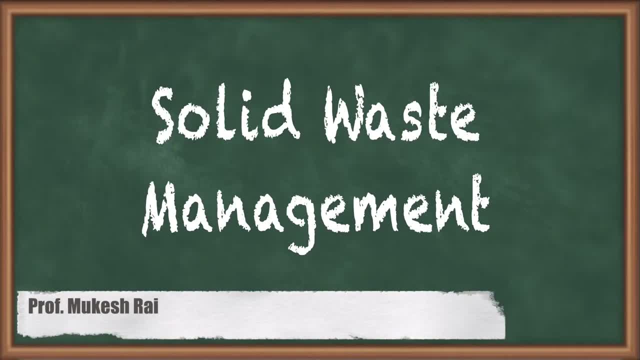 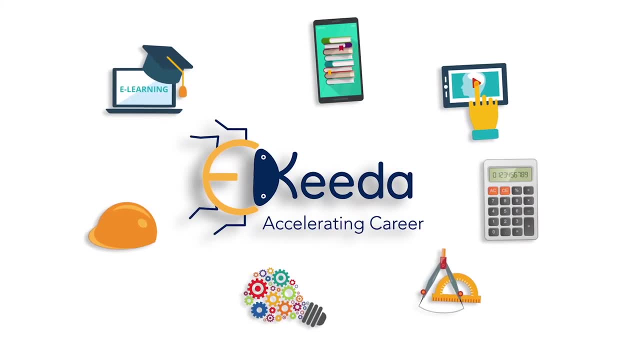 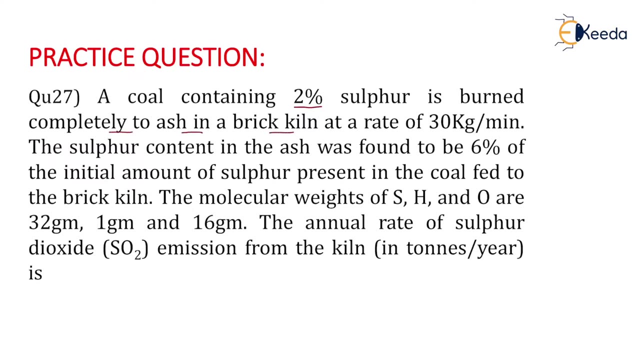 Hello students, today we are going to discuss the previous year gate question. A coal containing 2% sulfur is burnt completely to ash in a brick kiln at the rate of 30 kg per minute. Now the sulfur content in the ash was found to be 6% of the initial amount of sulfur. 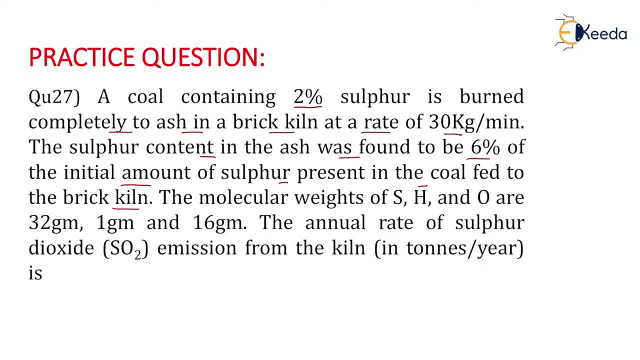 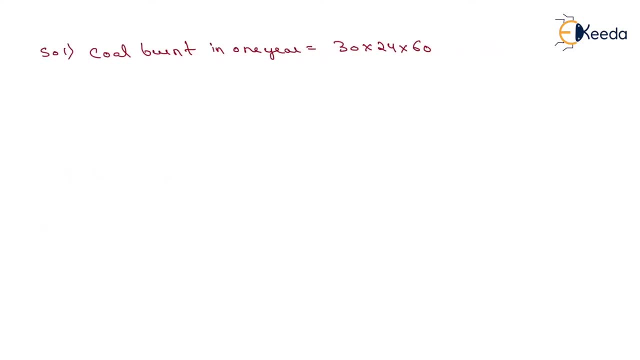 present in the coal fed to the brick kiln. Now the molecular weights of sulfur hydrogen oxygen are given as 32g, 1g and 16g. We need to compute the annual rate of sulfur dioxide emission from the kiln in tons per year. Now the coal burnt in one year is given as 30 x 24 x 60 x 365, because it 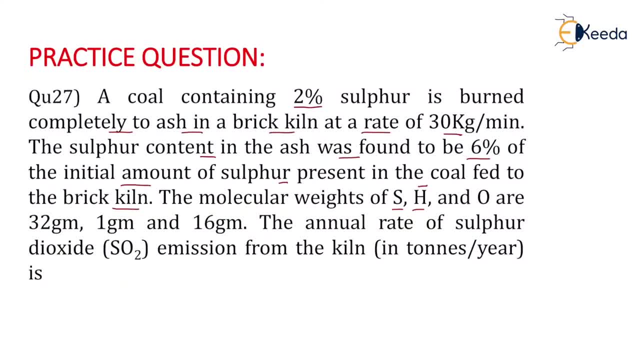 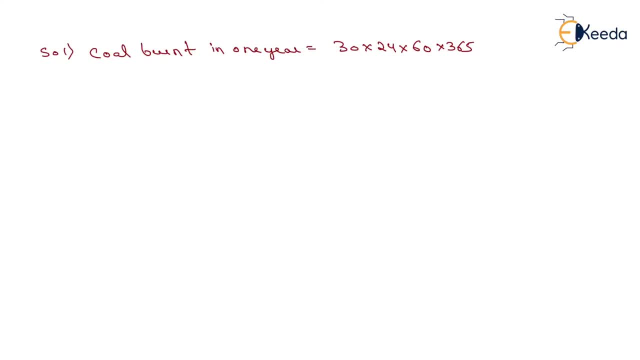 is given in the question that the coal is burnt at the rate of 30 kg per minute. But we want this in one year basis, so we had converted this kg per minute into per year basis. so we had multiplied with 24 x 60 x 365, it will be equals to 1.5768 x 10, to the power 7 kg, So the total coal burnt in. 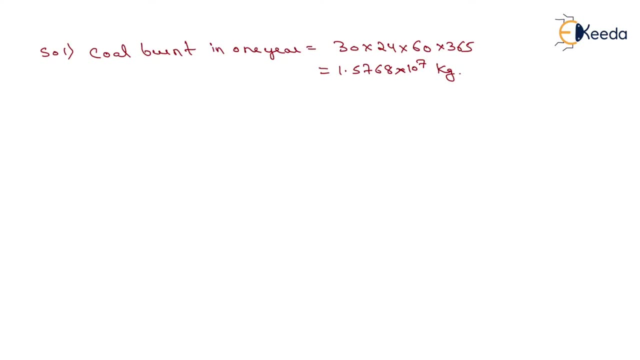 one year will be equals to 1.5768 x 10 to the power 7 kg. Now the sulfur content in the coal that will be present. okay, now the sulfur content in coal, it will be equals to what will be equal to 1.5768 x 10 to the power 7 kg. So the total coal burnt in one year it will be: 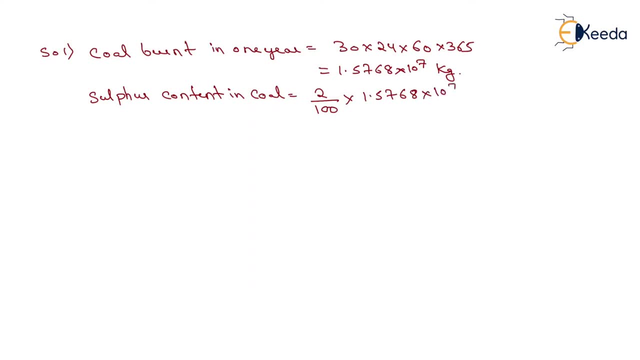 equals to 1.5768 x 10, to the power, 7 kg. After solving this, you will have the value as 315360 kg per year, and if you convert this value into 10, it will be equals to 315.360 tons per year. okay, that will be the total sulfur containing in the coal on per year basis, which we 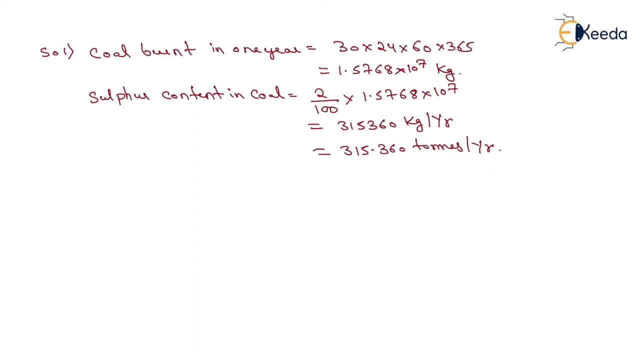 will be equal to 315.360 tons per year. now this whole content in ash, now the sulfur content in ash, it will be equal to what? 6 or the total sulfur content. so it will be equals to 6 divided by 100 into 315.360. it will be equals to what? 18.92 tons per year. that will be the sulfur content in ash. okay. 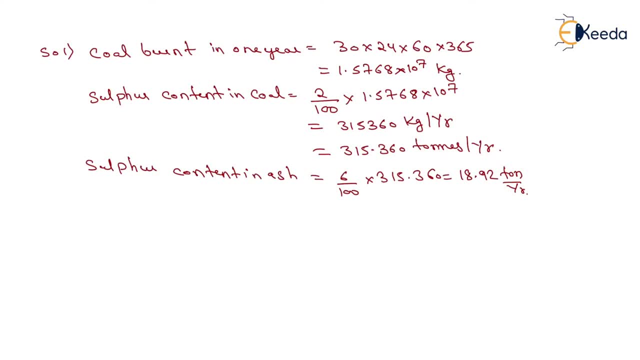 Now, how much amount of sulfur is converted, total in years? well, we will have to concentrate on�로 package, soil protection Happiness if you want to give any kind of이 to SO2. now we need to compute here: sulfur converted to SO2. sulfur converted to SO2, it will 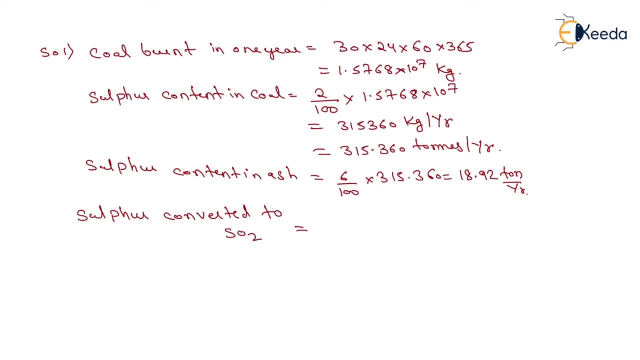 be the difference of total sulfur minus sulfur content in ash. so we just write it as 315.360 minus 18.92. it will be equals to 296.44 ton per year. okay, that will be the sulfur converted to SO2. now we know the reaction. that is, S plus O2 will be equals to what SO2. okay, now from here. 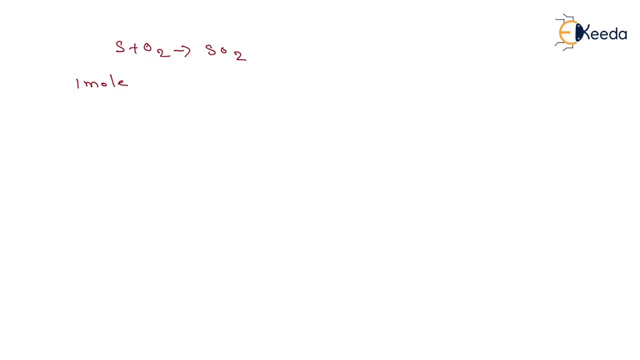 we know the value, that is, one mole of sulfur will require how much mole of SO2 it will be equals to one mole of SO2. so we just put the value of molecular weight as well as the atomic weight. so the atomic weight of sulfur will be given, as 32 gram of sulfur will be equals to 64 grams. 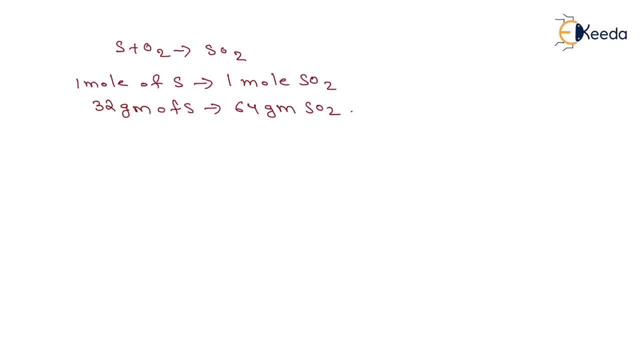 of SO2. okay, now from this we can determine that for 296.44 ton of sulfur per year, what will be the total amount of sulfur dioxide in ton per year? it will be equals to 64 into 296.44. divided by 32, it will be equals to 592.88 ton per year. it means that for the sulfur content of 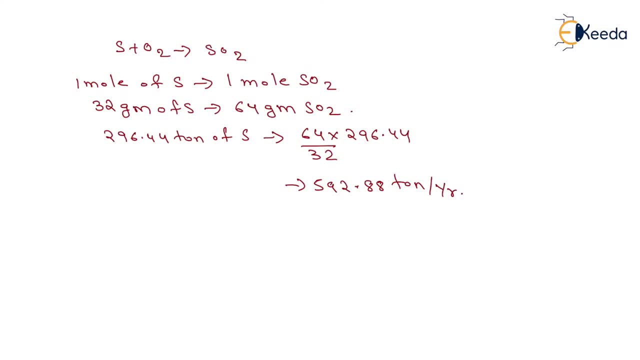 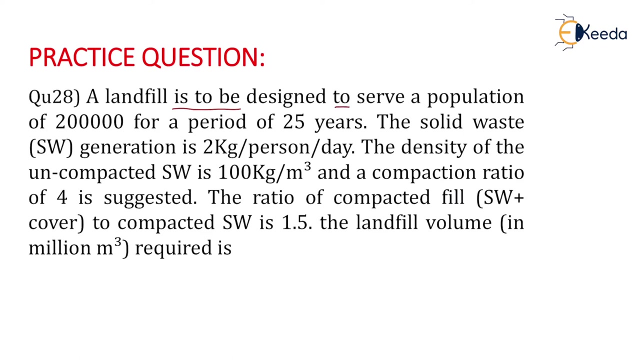 296.44. the SO2 quantity will be 592.88 ton per year. that will be the complete solution of this question. okay, students, now we can move to the next question, that is, a landfill is to be designed to serve a population of two lakhs? okay, for a period of 25 year, it means that population is given and 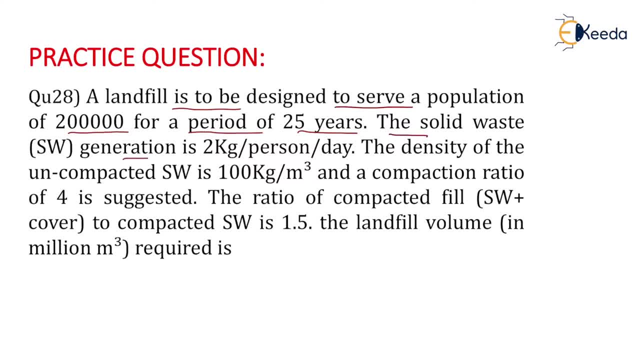 the number of year is also given. now the solid waste generation is two kg per year and the per person per day. it means that the per capita solid waste generation is given as 2 kg. okay, now the density of uncompacted solid waste is given as 100 kg per meter cube. it means that a 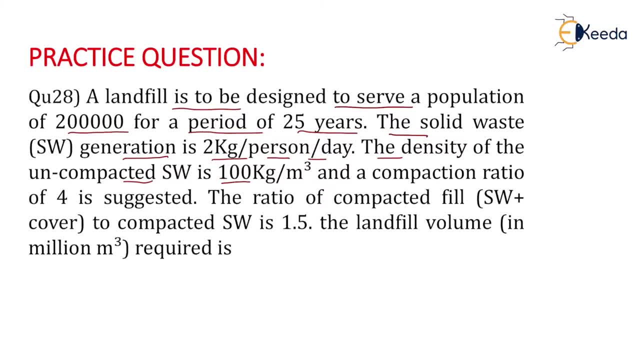 density of uncompacted solid waste is given as 100 kg per meter cube and a compaction ratio of 4 is suggested. it means that the volume before compaction upon volume of after compaction is given as 4, now the ratio of compacted fill, that is. 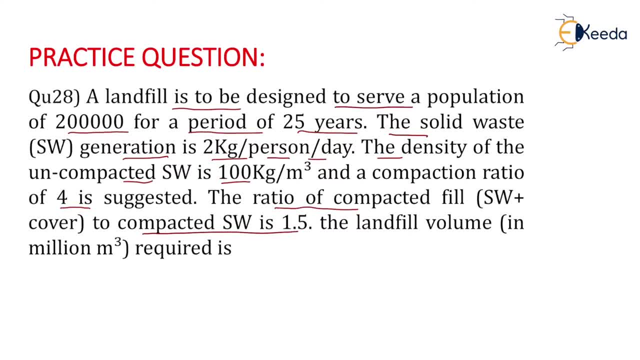 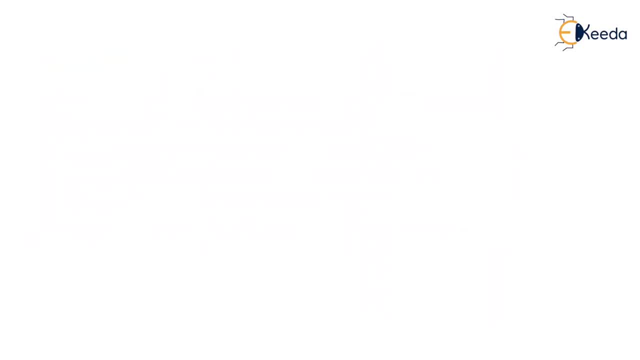 solid waste plus cover to the compacted solid waste is given as 1.5. now we need to compute the landfill volume in million meter cube required is okay, so we start the numerical by just writing the given quantities as population, which will be equals to 2 lakhs, okay, and the number of year is: 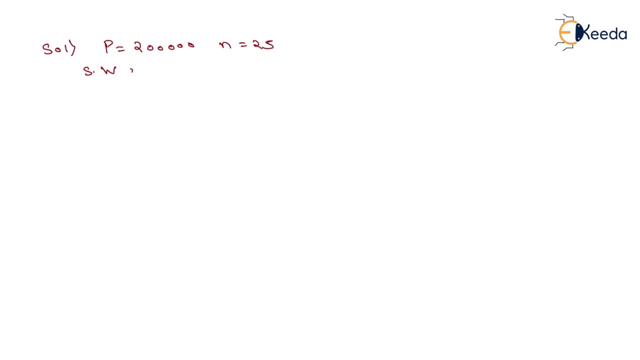 given as 25: solid waste generation by one person. solid waste generation by one person. it will be equals to 2 kg per day. so we need to compute the landfill volume in million meter cube required is. so we just write it as: solid waste generation by one person equals to 2 kg per capita per day. okay, 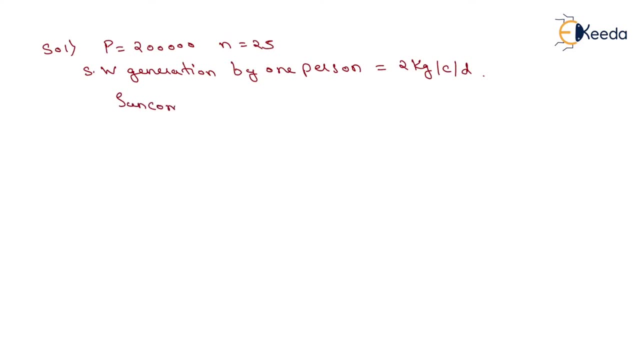 now the density of uncompacted solid waste is already given in the quotient, which will be equals to what it will be equals to 100 kg per meter cube. now the compaction ratio is also given, that is, the compaction ratio will be equals to what it will be the volume of solid waste before. 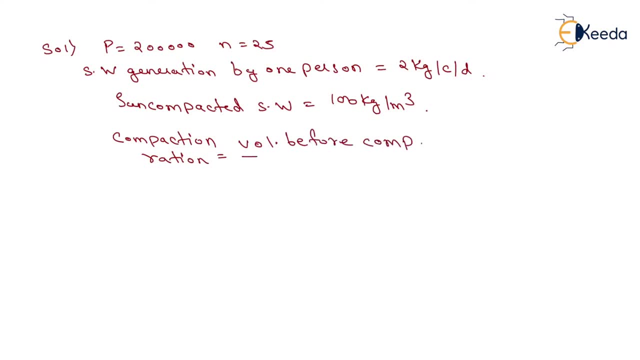 compaction upon volume of solid waste after compaction. okay, so it will be given as what it will be equals to 4. now we want to compute the total solid waste generated per day. now the total solid waste generated per day will be equals to what? solid waste generated per day will be equals to what? 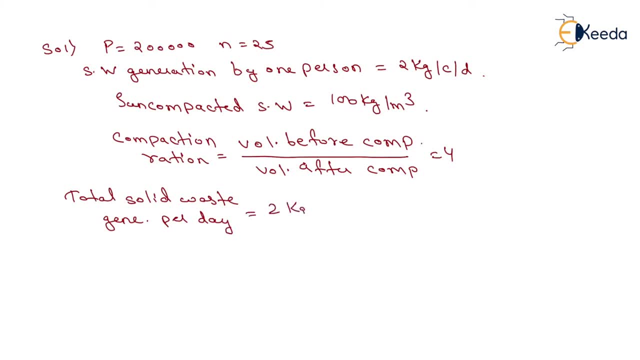 we need to multiply the per capita solid waste generation by the total capita which will be present in that city, which will be equals to 2 lakhs. okay, now, multiplying it, it will be equals to 4 into 10, to the power 5 kg per day. it means that the total solid waste produced, or 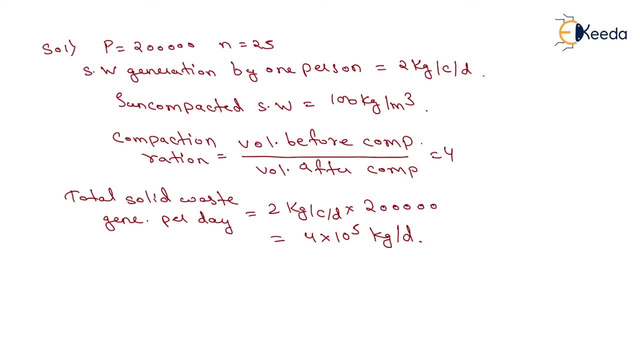 generated in one day will be equals to 4 into 10 to the power: 5 kg per day. now we want this for 25 years. so total solid waste generated in 25 years: total solid waste generated in 25 year. now we need to multiply this by 4 into 10 to the power: 5 kg per day. but we need to compute this in per day basis. 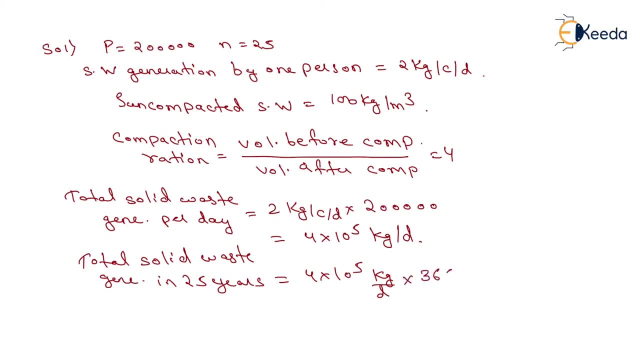 or for 25 years. so we need to multiply here 365 days. so we had converted this on kg per year basis and we need to multiply here 25, so it will be equals to what 365 triple zero into 10 to the power: 5 kg, that will be the total solid waste generated in 25 year. okay, 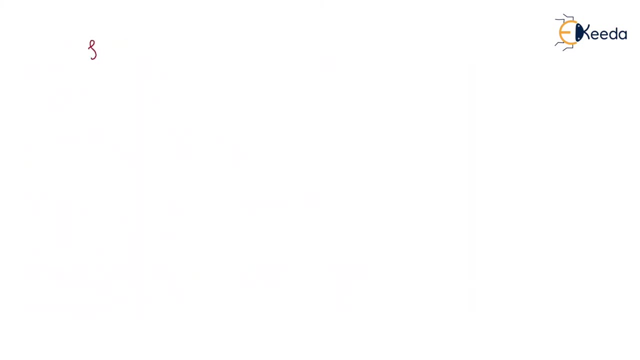 now we know that density of uncompacted solid waste will be equals to what it will be the ratio of weight by volume, and the weight is already given. we had computed it 365 double zero into 10, to the power, 5 kg. and we need to compute the volume of uncompacted solid waste because 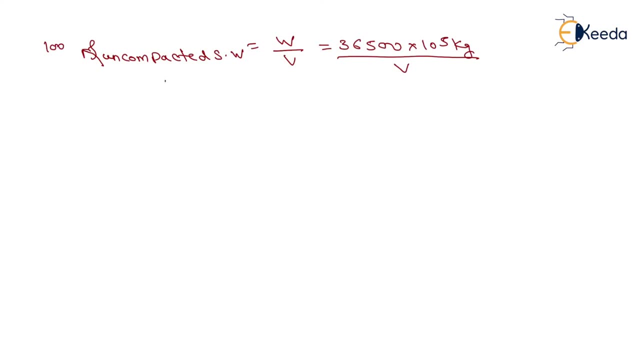 the density is given as 100 kg per meter cube. now the volume of uncompacted solid waste coming from this equation will be equals to what it will be equals to 365 into 10, to the power, 5 meter cube. okay, now we know that the compaction ratio is already given. 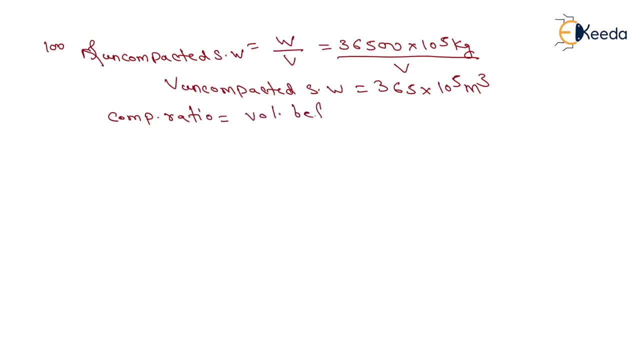 compaction ratio will be equals to volume before compaction upon volume after compaction. okay, now the compaction ratio is already given, which will be equals to what? 4- and we had computed the volume before compaction- it will be equals to 365 into 10 to. 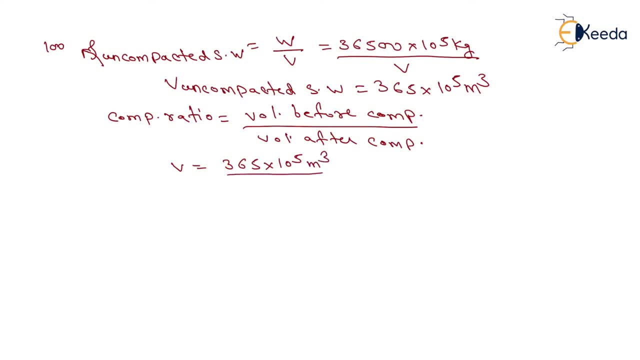 the power 5 meter cube. now we need to compute the volume after compaction, which will be indicated by v dash. okay, it is already given that is 4. now we from this we can compute the value of v dash, which will be equals to what 9125 triple zero meter cube. that will be the volume after compaction. okay, 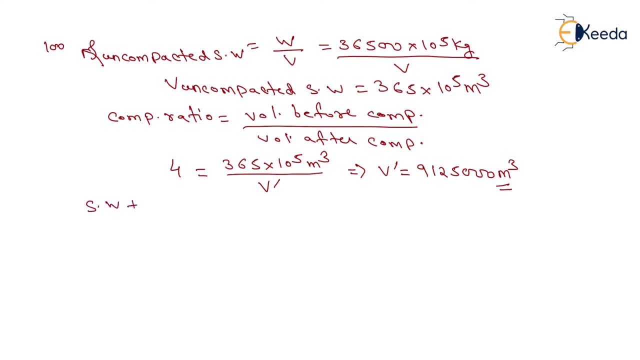 okay, now a ratio is given, that is, the volume of solid waste plus cover divided by volume of solid waste. it will be equals to what? 1.5? now we need to compute the total volume, which will be equals to volume of compacted solid waste plus volume of cover, which will be equals to 1.5, into solid waste, or the volume of solid 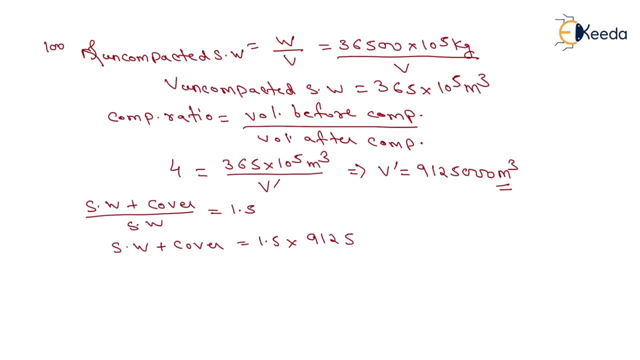 waste after compaction. so we just need to multiply it by 9125 triple zero, it will be equals to 13.6875 into 10, to the power 6 meter cube. so it will be equals to what 13.6875 million meter cube. 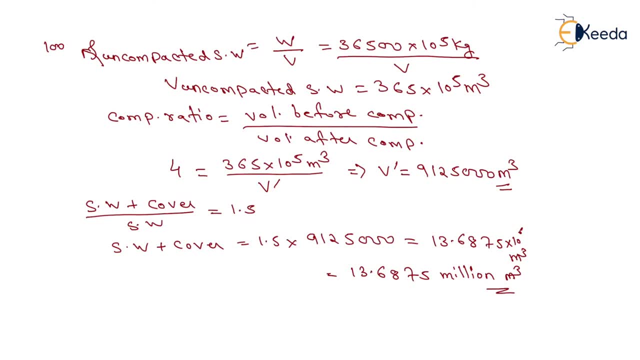 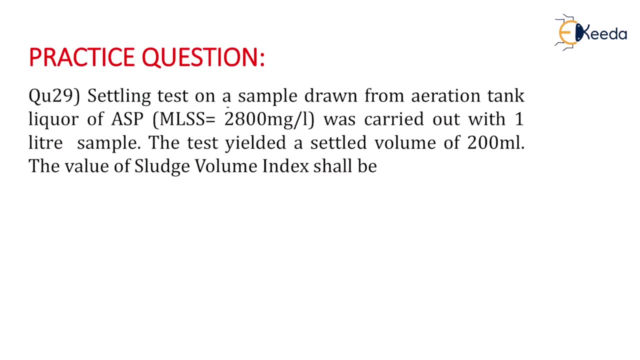 okay, that will be the complete volume of solid waste plus cover, which will be equals to what? 13.6875 million meter cube. now the next question is given as settling test on a sample drawn from aeration tank liqueur of activated sludge process, that is, mlss is equals to 2800 milligram per liter, was carried. 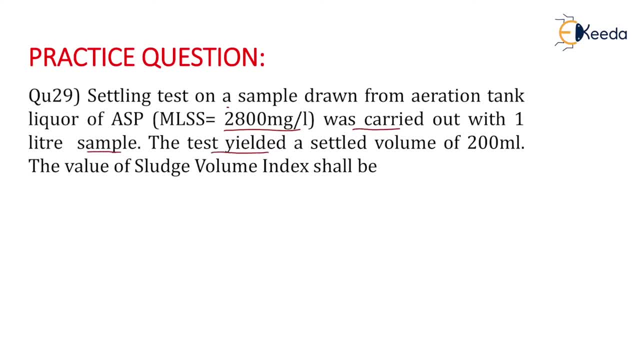 out with one liter sample. now the test yielded a settled volume of 200 ml. the value of sludge volume index shall be: now we know the formula of sludge volume index: it will be the ratio of volume of settled sludge divided by weight of suspended solids present in the mlss in 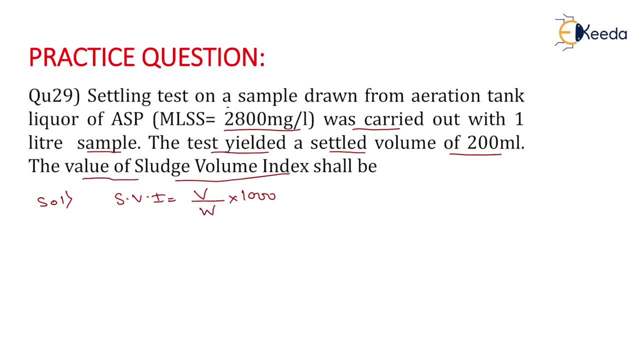 2004 computation of sludge volume index in milliliter per gram. now we have the volume as equals to 200 ml, and we have the value of mlss, which will be equals to 2800 into 1000 and the value will be comes out. 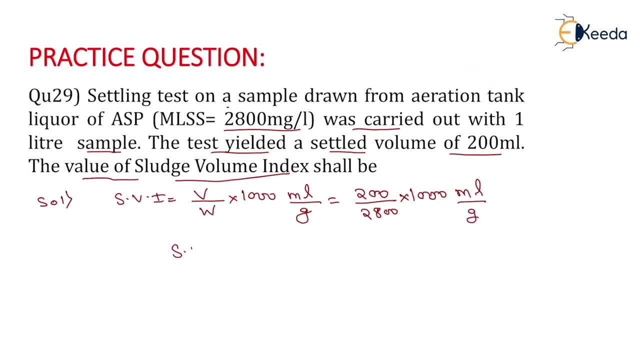 in milliliter per gram and, after solving this, we will have the value of sludge volume index, which will be equals to 71.43 milliliter per gram. that will be the sludge volume index for this question. now we can move to the next question. okay, 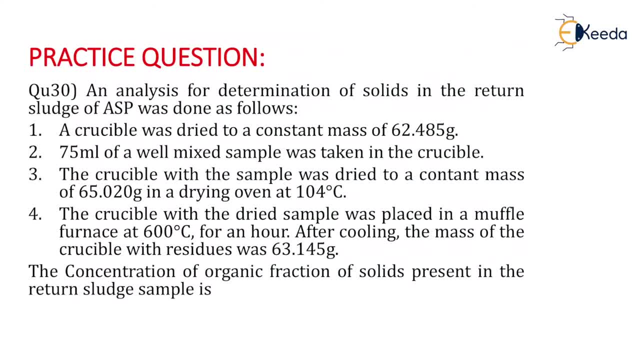 now the next question is given as an analysis for determination of solid in the written sludge, of activated sludge, process was done as follows: a crucible was dried to a constant mass of 62.48. now 75 ml of well mixed sample was taken in the crucible. the crucible with the sample was dried to a constant mass of 65.2. Seite table. Here we go. IT is shown to beガلا utopía valvularic as 화장liata mass of gaanata. Now, 75 ml of well mixed sample was taken in the crucible. that prayer table is also gotten as consistent mass of 62.. A crucible with sample과 60.22mmM is nothing special. a constant mass of 64.22ml is nothing special. The crucible came under warming temperature of 95 degrees and from there there is no lack of stress or Nov. 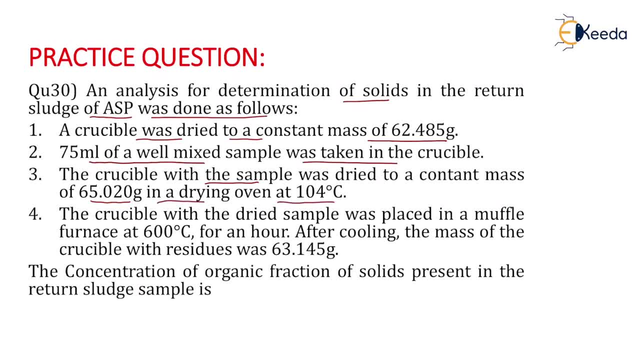 gram in a drying oven at 104 degrees celsius. now. the crucible with the dried sample was placed in a muffle furnace at 600 degrees celsius for an hour after cooling. the mass of crucible with residue was 63.145 gram now. the concentration of organic fraction of solid present in the 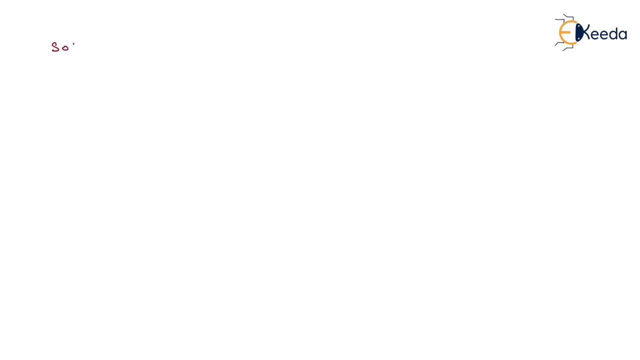 written sample is okay. now, firstly, what we have. we have the weight of sample. weight of sample of 105 degrees celsius or 104 degrees celsius. weight of sample of 104 degrees celsius: it will be equals to 65.02 gram. now we have the weight of sample of 600 or at 600 degrees celsius. okay, it will be. 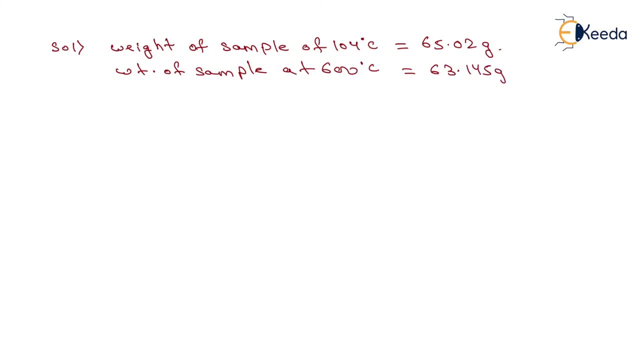 equals to what? 63.145 gram? now we have the weight of sample at 104 degrees celsius, which will be equals to 65.02 gram, and we have the weight of sample at 600 degrees celsius, which will be equal to 63.145 gram, which is already given in the question. now all the organic. 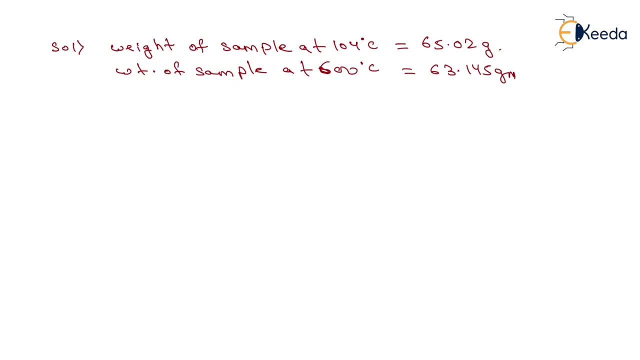 matter will be converted into carbon dioxide, water vapor and other gases at 600 degrees celsius. okay, now, the concentration of the cosine of. okay, now, the concentration of the cosine of Nazi gas. ど nutritious matrix and no waste of money. first of all, I would never assemble zero kilogram number of which are waste, which are 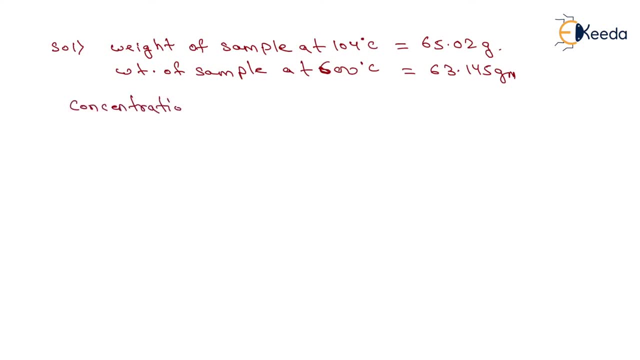 this is what you should all I said earlier from the first. I just do the argument in sense of concentration of organic fraction. now, the concentration of organic fraction of solid will be equals to what organic fraction of solid will be equals to what it will be the ratio of? 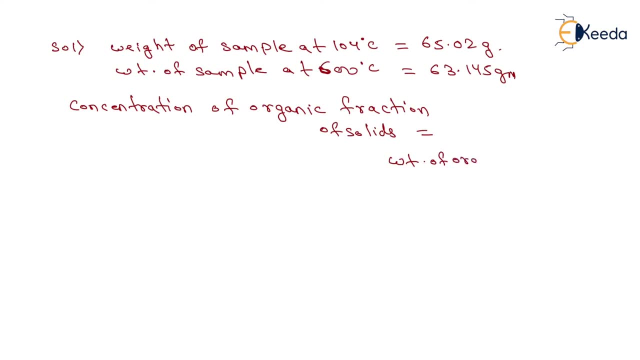 weight of organic fraction. weight of organic fraction divided by volume of sample, which is already given in the question, that is, volume of sample. now, what will be the weight of organic fraction? it will be the difference of 65.02 minus 63.145 divided by 75, and we need to compute this. 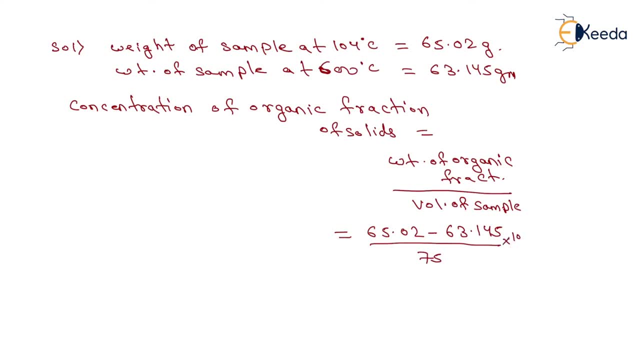 value in terms of milligram per liter, for which we need to convert this by 10 to the power 3, upon 10 to the power minus 3. after solving this, you will have the value of 25 000 thousand milligram per liter. that will be the concentration of organic fraction of solid.